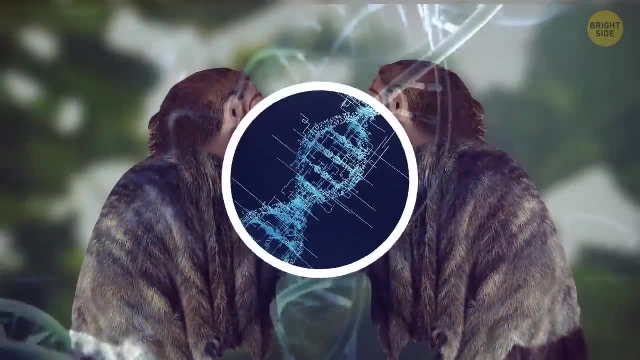 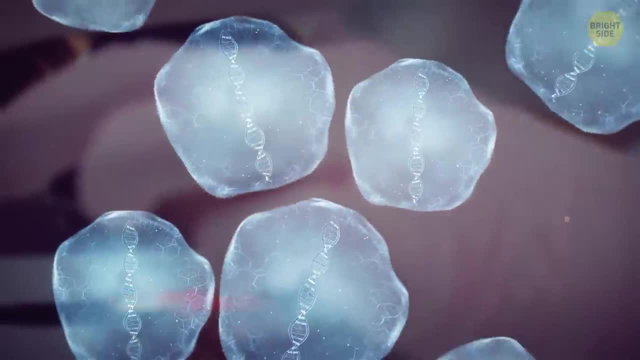 Now you know how things go when folks live near each other. Some genetic mixing was bound to happen. The evidence: A dash of Neanderthal DNA which was found in modern folks. Now this is where the plot thickens. Scientists thought that, since Neanderthals never lived in Africa, 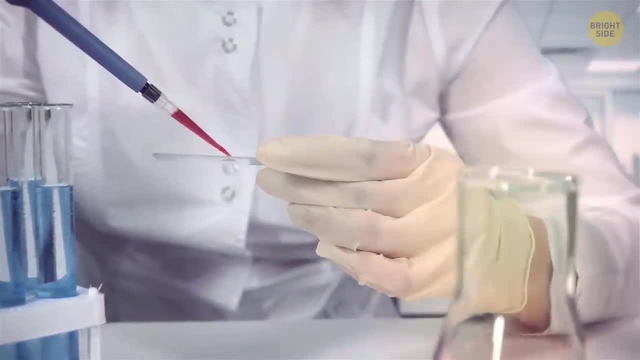 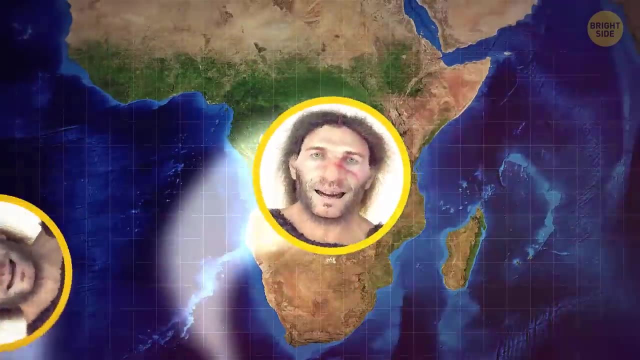 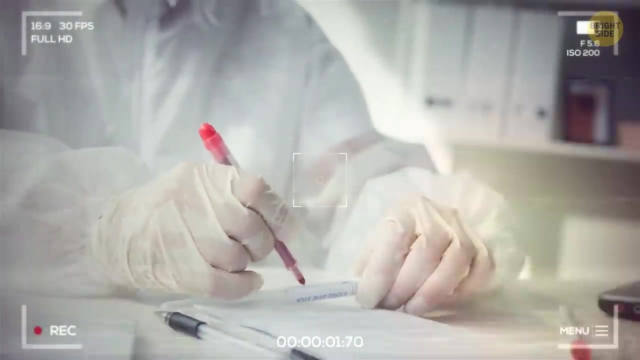 their DNA wouldn't be found in modern African populations. Well, it turns out that African people have about 0.5% Neanderthal DNA too. This doesn't mean our Neanderthal relatives simply teleported through African territories without leaving any trace behind. What this discovery actually implies is that early humans 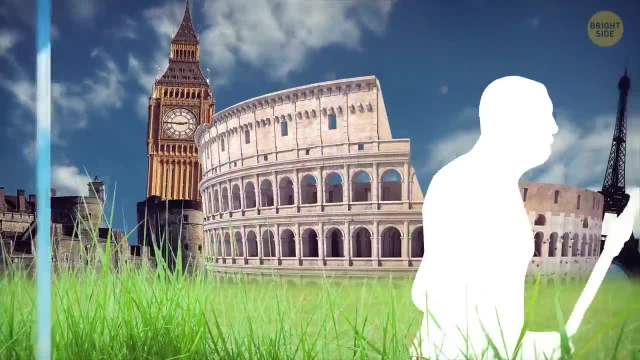 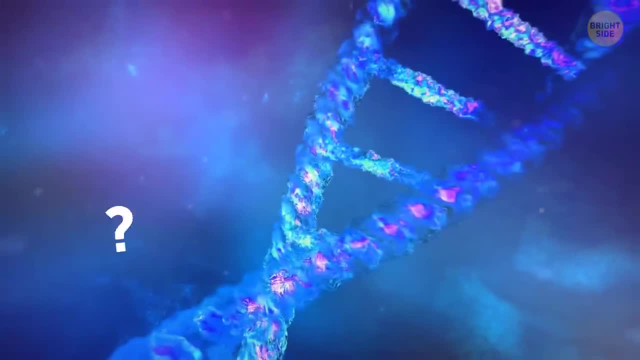 might have visited Europe, mixed their genetic material with that of Neanderthals, after which they returned to Africa. This is a very interesting discovery. It's a very interesting discovery. That's a lot of migration. How did we stumble upon that Neanderthal DNA these days, you might wonder. 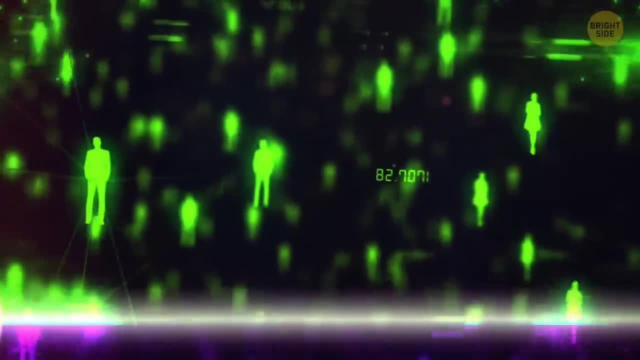 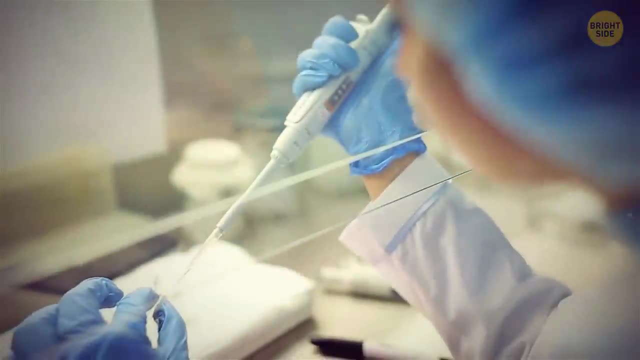 Well, scientists gathered thousands of people from all around the world. Participants came from places like East Asia, Europe, South Asia, America and Africa. Percentages may vary, sure, but around 20% of the good old Neanderthal DNA is still found in US modern folks. Sure. the average Joe only carries about 2% of that caveman swagger. If you're from certain places or families that have a lot of Neanderthal DNA, you might be able to find a lot of Neanderthal DNA, But you're looking at 3% tops. Is there anything in particular that we share with our long-gone humanoid cousins? As it turns out, our Neanderthal ancestors gifted us more than just their company for some thousands of years. They also passed down the incredible legacy of… their noses. 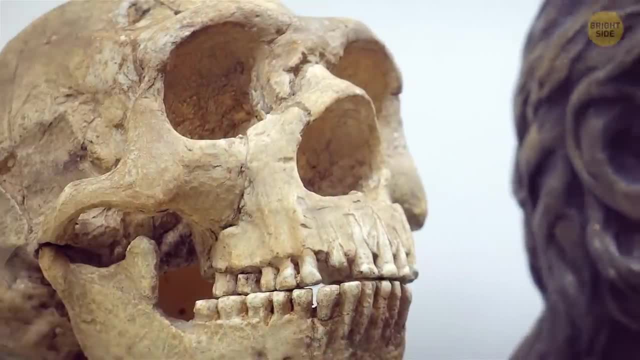 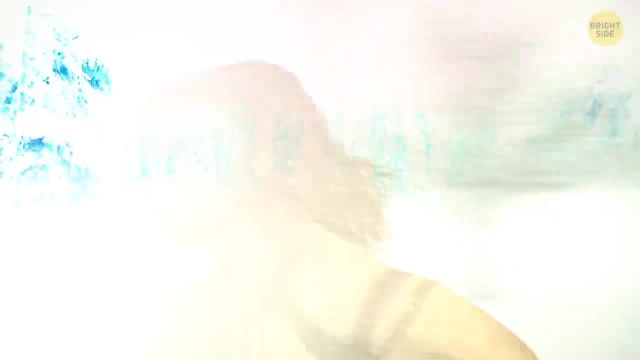 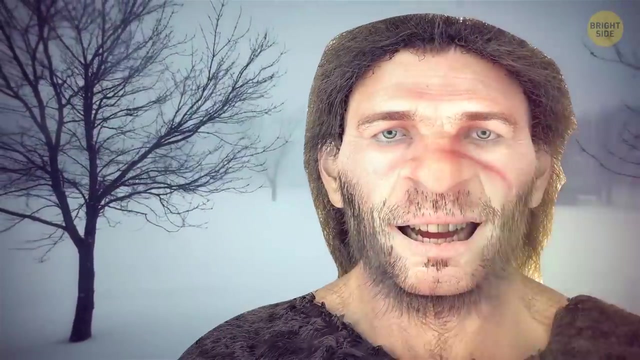 were also quite the asset in chilly climates, The icicle-dripping, teeth-chattering kind of cold where your breath could freeze before it leaves your lips. During those days, the Neanderthal noses worked as personal heaters, warming and humidifying the cold, dry air. they 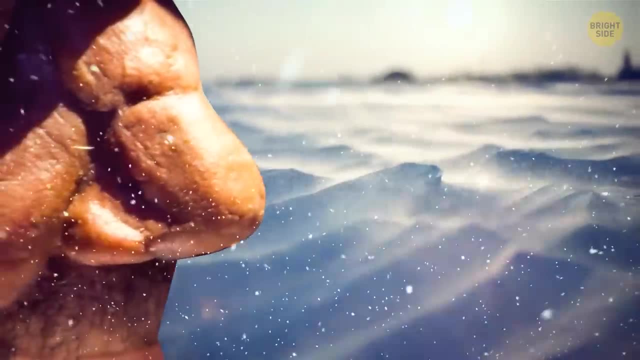 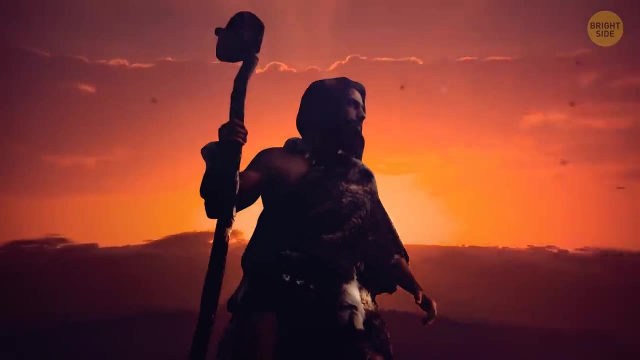 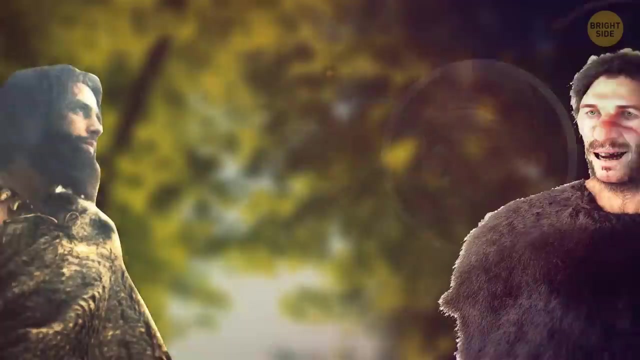 inhaled. For that kind of extreme weather, these impressive nasal skyscrapers turned out to be quite handy. When our Homo sapiens ancestors decided to leave the sunny savannas of Africa for a spot of frostbite up in Eurasia, they bumped into the Neanderthals. This encounter resulted. 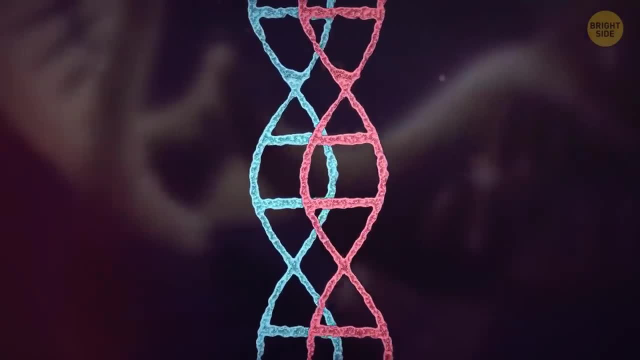 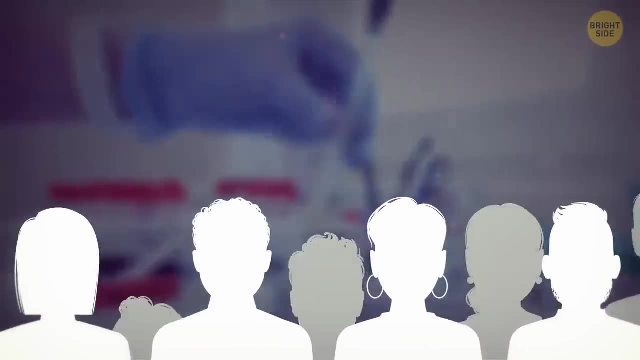 in not just an exchange of pleasantries, but also an exchange of genes that coded for larger noses. This newfound genetic nugget was discovered by scientists who dug deep into the DNA of over 6,000 volunteers To complete the study. these scientists meticulously compared. 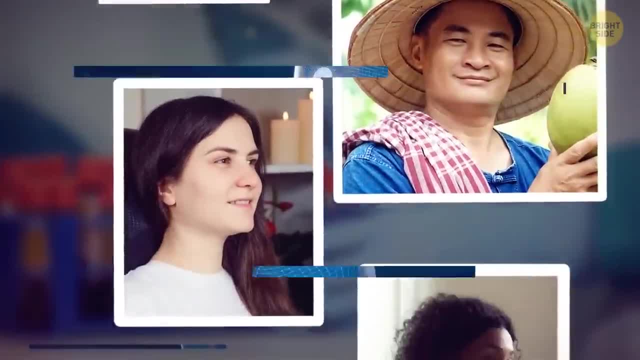 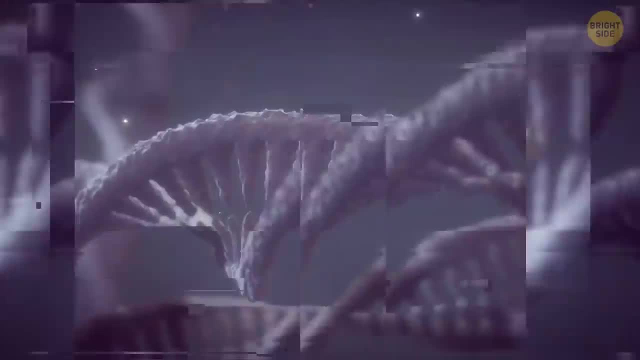 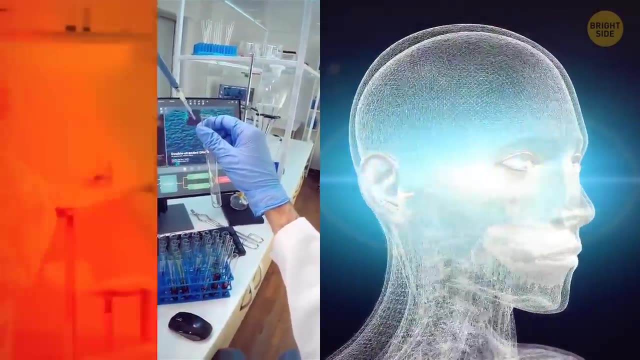 this genetic data to snapshots of the volunteers' faces. They measured the distances between various points on each face, height of the volunteer's nose bridges. They then played a game of spot the genetic marker to identify if certain facial traits were linked with specific genes. 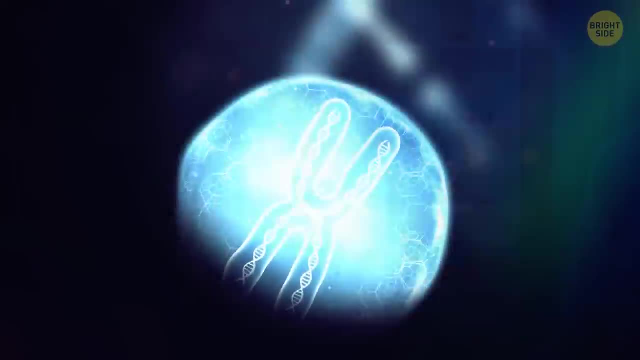 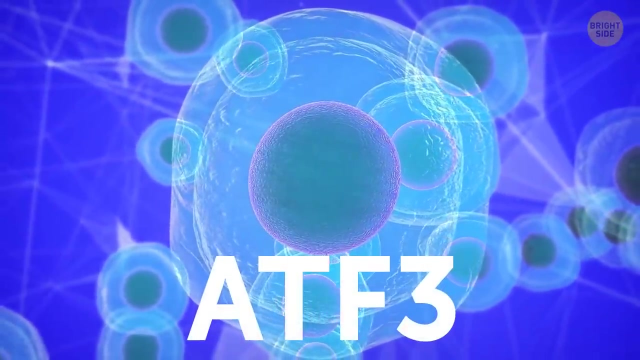 By the end of this exciting chase, they hit the jackpot: 33 shiny new genome areas were linked to facial features. One standout gene, named ATF3, was traced back to our Neanderthal ancestors and seemed to be the maestro of controlling nose height. 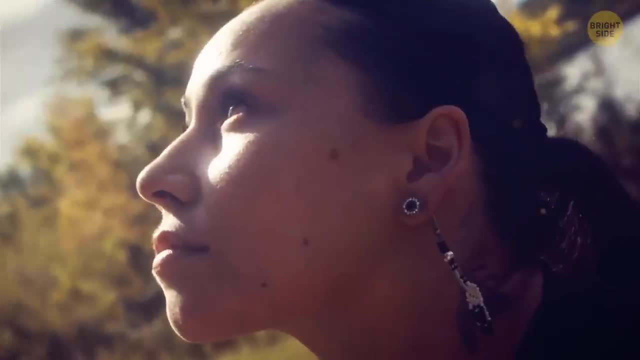 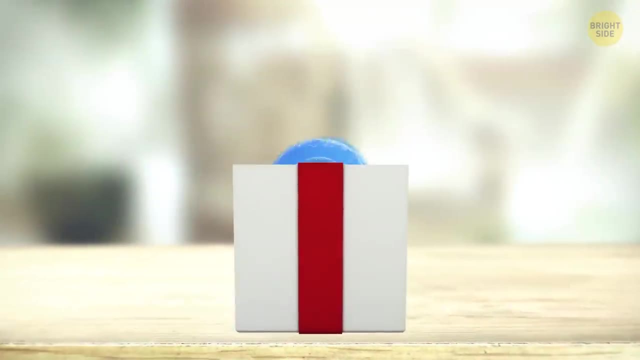 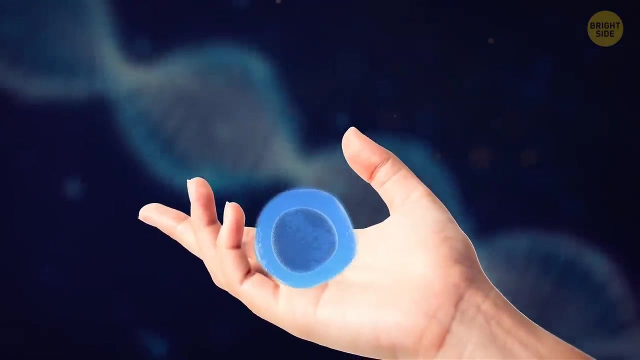 Participants with Native American ancestry had Neanderthal hand-me-downs in this gene, contributing to their taller noses. Think of the ATF3 gene as a Neanderthal housewarming gift to us humans as we stepped into colder climates from Africa. Interestingly, this isn't the first time our ancestors have played Pass the Gene. 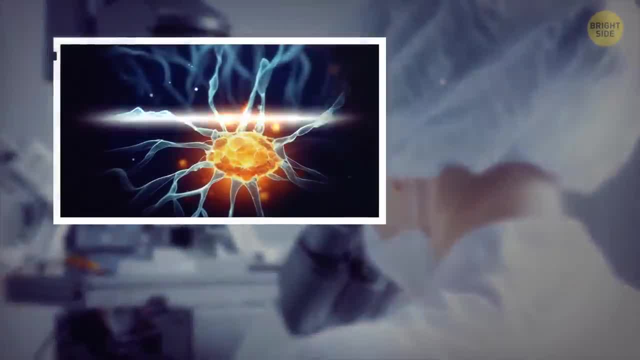 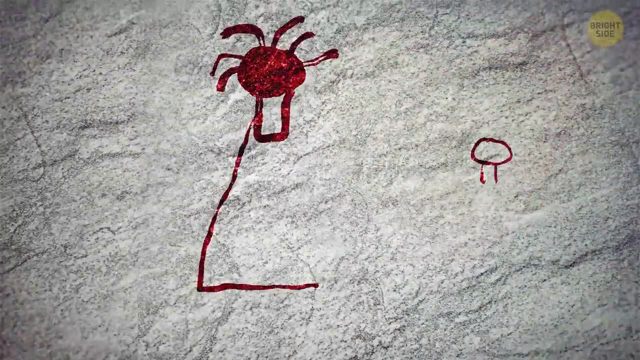 Back in 2021, the same research team uncovered a gene influencing lip shape called TBX15.. This gene was a little love note from the Denisovans, another set of our ancient relatives who lived in Asia and went extinct around 30,000 years ago. 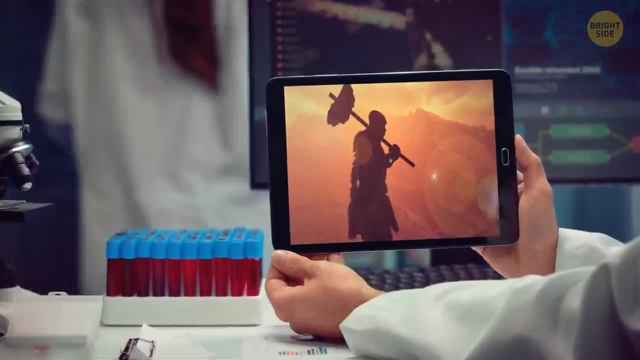 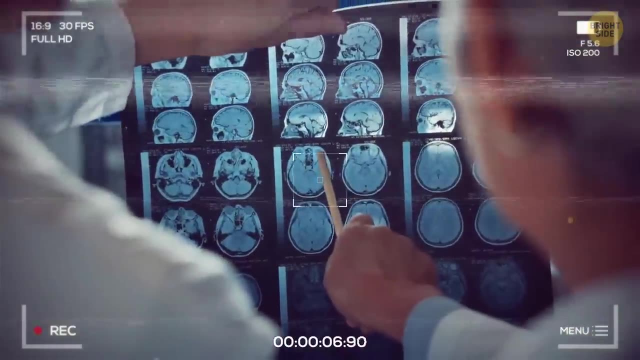 Another part of the scientific community believes our Neanderthal buddies had this weird genetic feature when it came to their brains. Is that why they didn't make it? Through this theory, it was suggested that US humans might owe our brainy edge to a 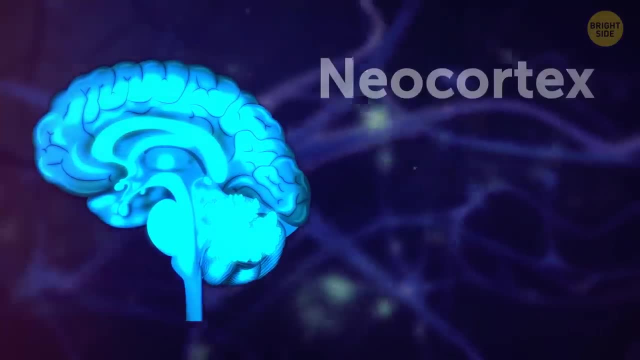 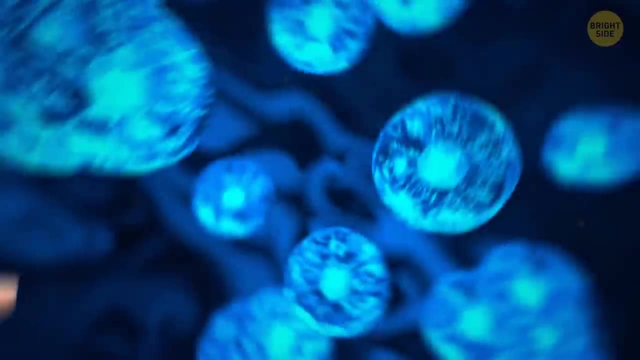 quirky gene mutation. This mutation gave our neocortex- that's the smarty pants part of the brain, a little population boom in the neuron department. This amazing gene of ours isn't all that different from the Neanderthal version. It's just one amino acid off. 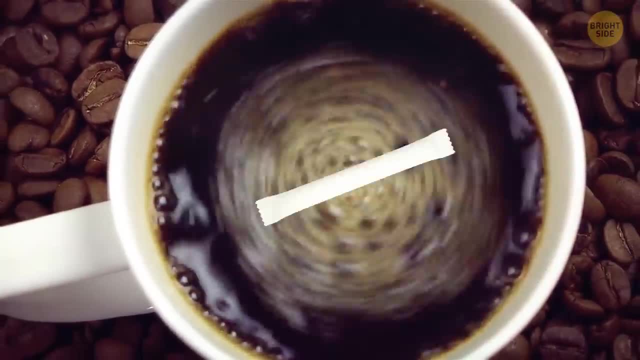 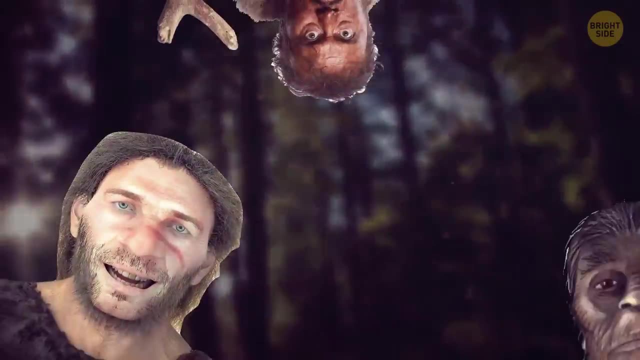 That's it, Just like ordering a coffee with one sugar instead of none. This tiny tweak is found in virtually all modern humans. Meanwhile, our extinct relatives, the Neanderthals, Denisovans and other primate pals all missed. 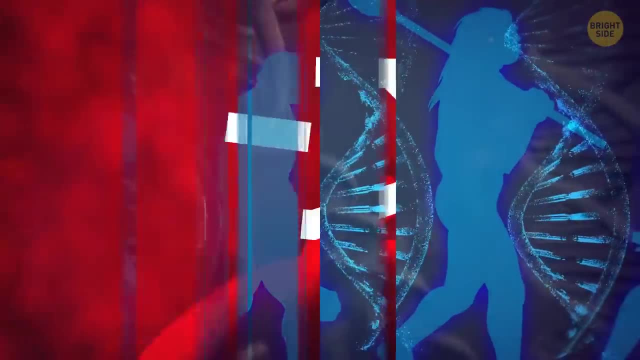 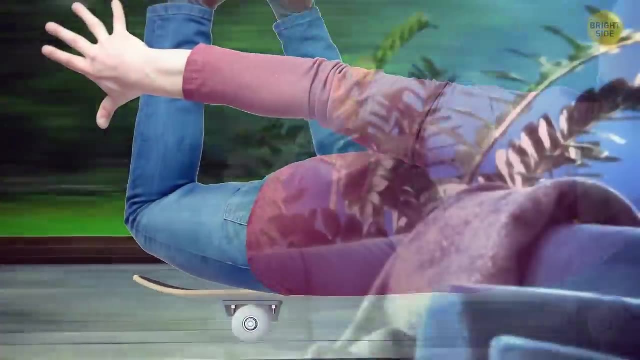 the mutation memo, at least according to the study. Now let's not get ahead of ourselves. Just because we have more neurons doesn't necessarily mean we're geniuses by comparison. But these results do suggest that we might have rewired the brain in a way that gave. 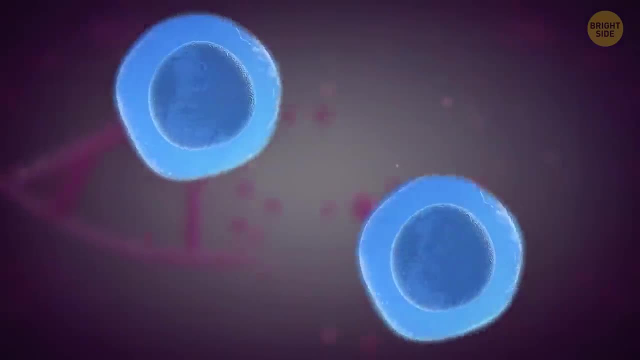 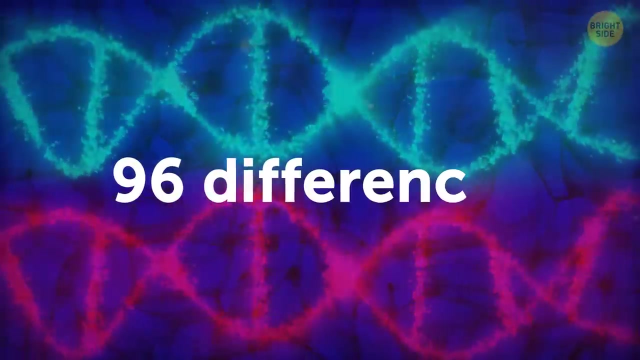 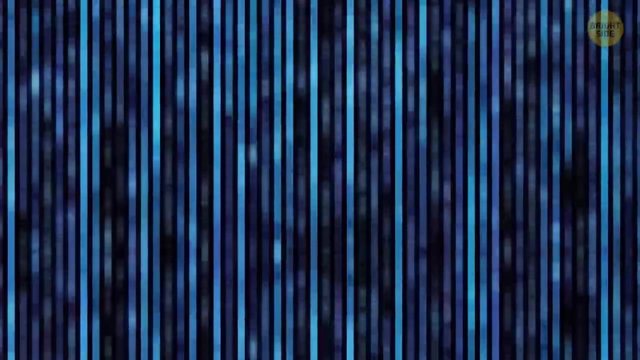 us a cognitive leg up. Also, it's not all about this lone amino acid difference. It's just a piece of the puzzle. Scientists have previously found a whopping 96 differences between our DNA and that of Neanderthals that could have potentially affected our different outcomes as species. 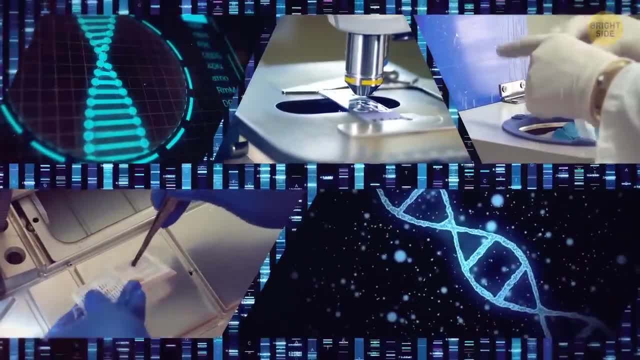 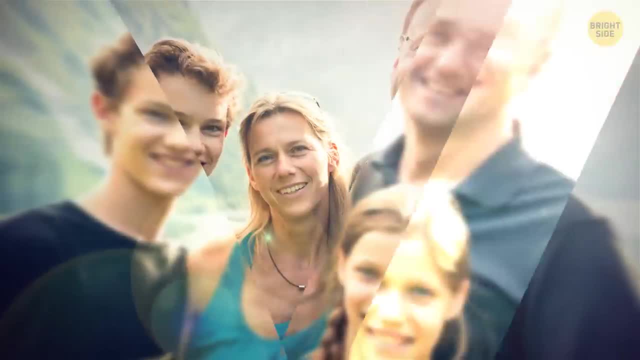 Studying Neanderthal DNA also gave us some insight into their relationships. In fact, we now have some solid evidence of what a Neanderthal family looked like, And, surprisingly, it's not really that different from ours. For this study, researchers gathered over a year and a half of DNA samples from the 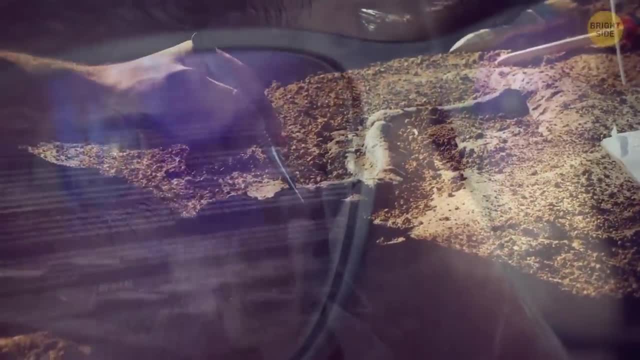 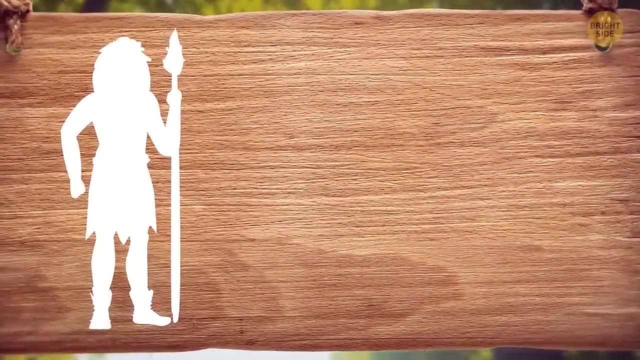 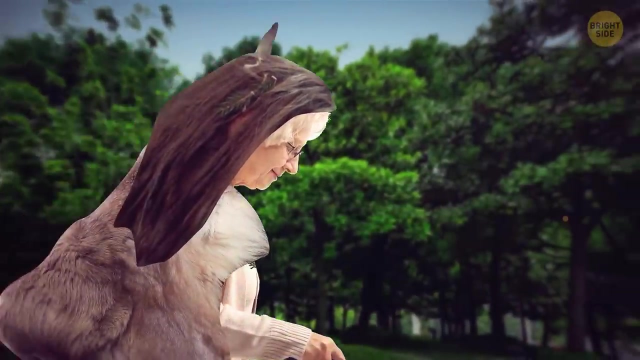 Neanderthal Archaeological Site located in Asia, They discovered that one particular family included a doting Neanderthal dad, his teen daughter and a sprightly young lad who was possibly their nephew or cousin. Part of the group was also an older female relative, maybe an aunt or granny. 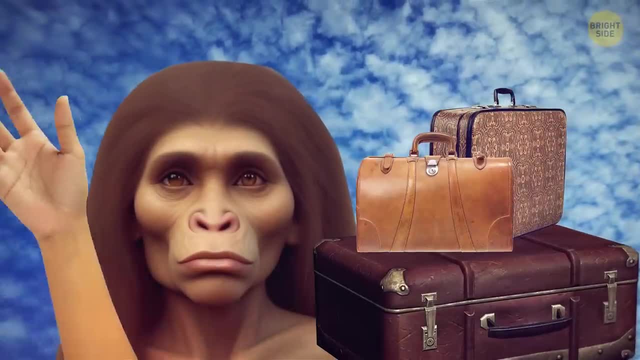 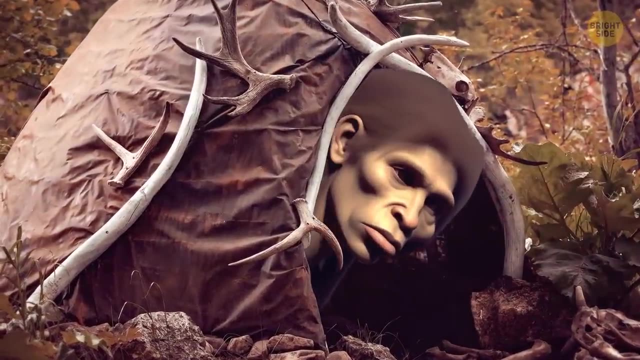 Now our young damsel would eventually pack her bags, wave a teary goodbye and leave her papa's home when she found Mr Right. Had she been a boy, like her young cousin, She would have been a happy homebody. But worry not, she wasn't stepping into a world of strangers. 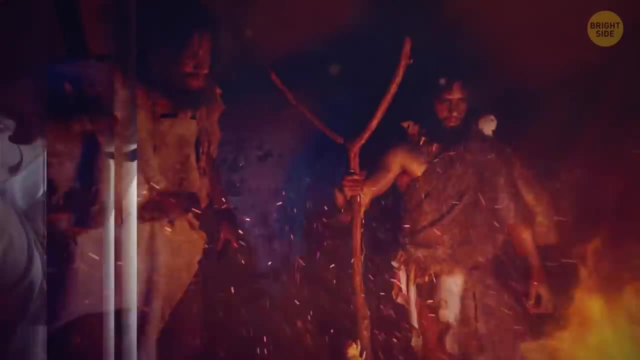 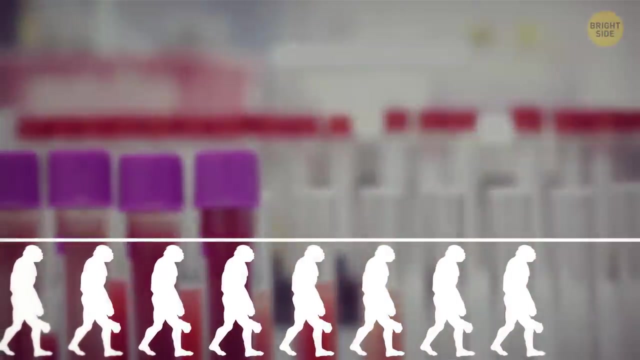 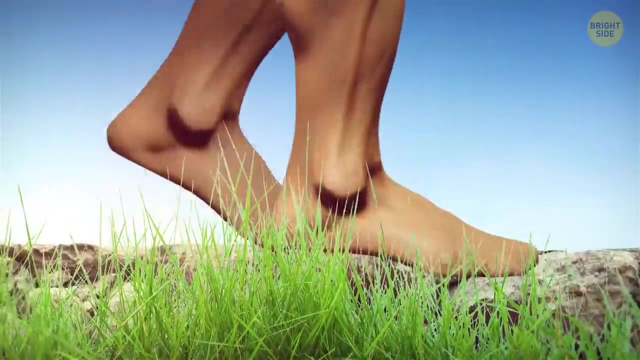 Her new community likely had some familiar, friendly faces, But how were scientists able to predict the ending of this story? By browsing through their gene pool, researchers were able to figure out that the Neanderthal social structure was patrilocal. What this means is that most female Neanderthals left their homes when choosing a partner. 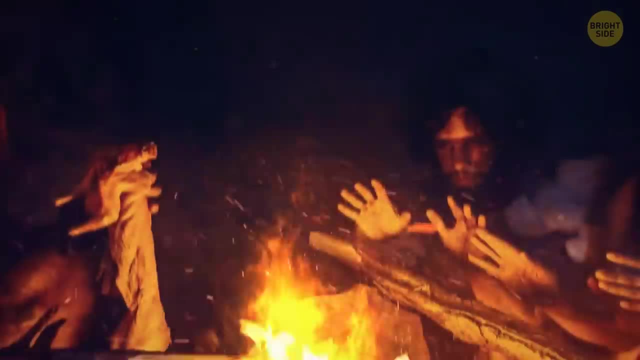 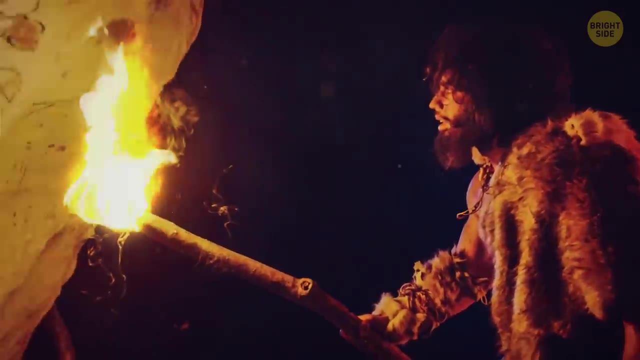 and started a new life with another family. The same researchers were able to figure out that the Neanderthal social structure was patrilocal. Research shows that our cave-dwelling clans likely weren't living in isolation either. Families living close by were probably visiting the same rock sampling areas to make their 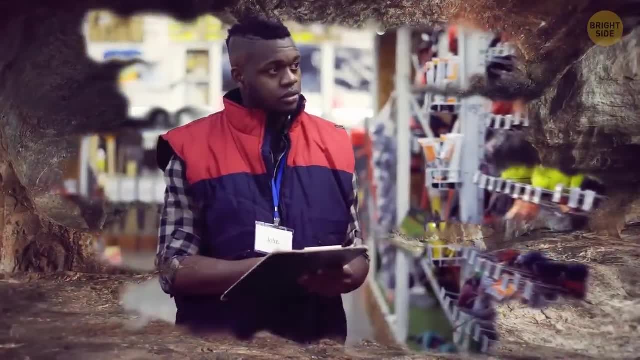 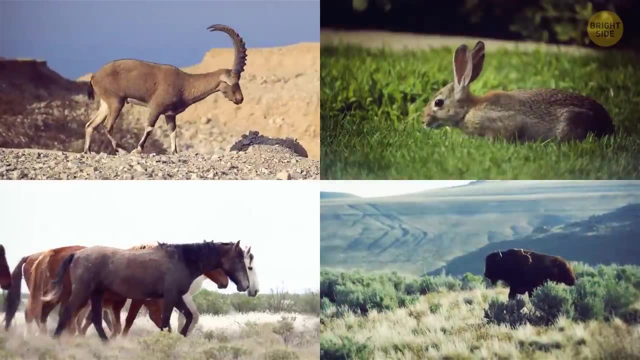 stone tools, the equivalent of a neighborhood hardware store, And when they weren't tooling around, they were busy hunting delicious meals like ibex, horses, bison and other wandering critters. Scientists, however, were careful to add that this ancient family portrait might not represent. 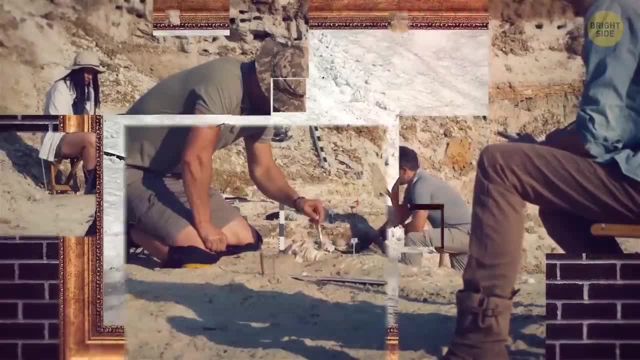 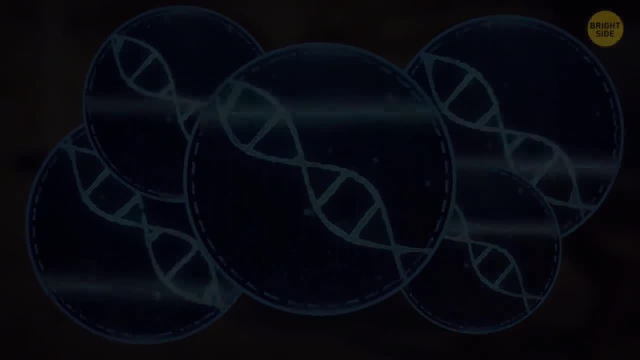 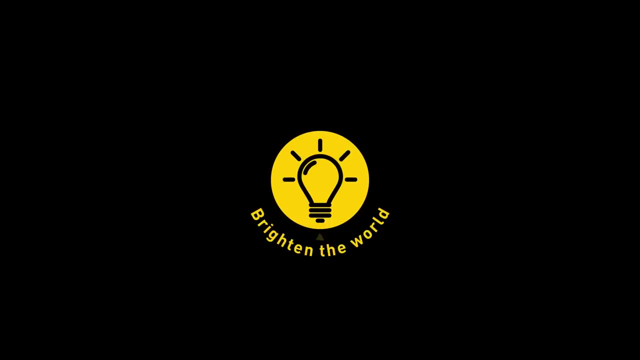 the full spectrum of Neanderthal social life. They've kindly asked future archaeologists To get more Neanderthal DNAs on the Ancestry websites.